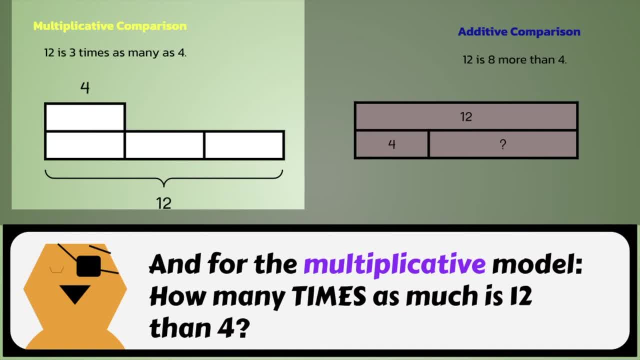 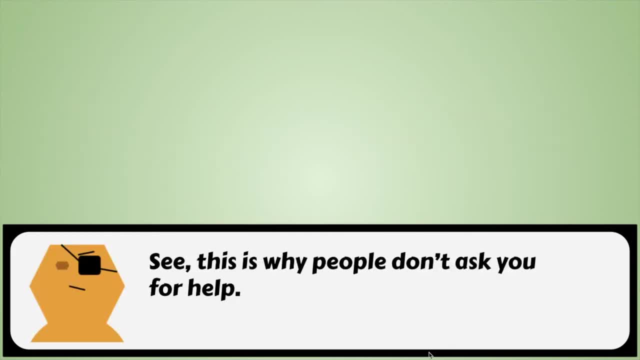 And for the multiplicative model, how many times as much as 12 than 4?? Hey, look at you pronouncing multiplicative correctly, See? this is why people don't ask you for help. Okay, okay, okay, Here's another one. 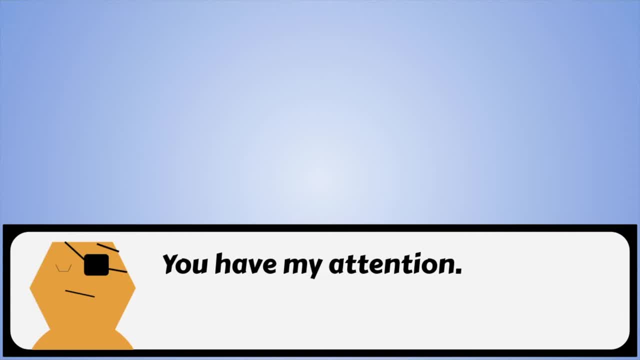 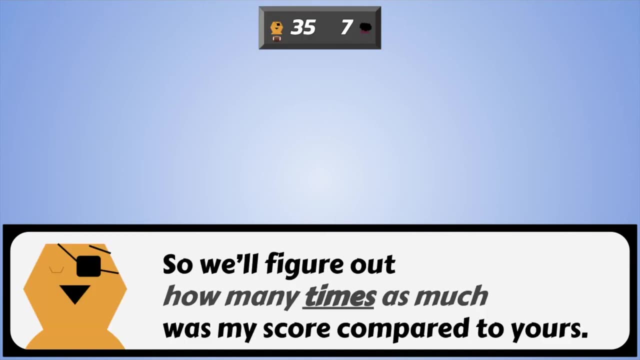 Let's use the score from our football game from yesterday. You have my attention. The final score was 35 to 7.. We can compare these numbers. I'm sorry, what was the score? The final score was 35 to 7.. Let's compare these numbers multiplicatively. 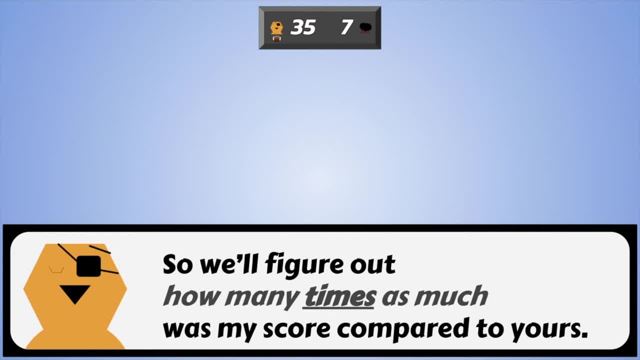 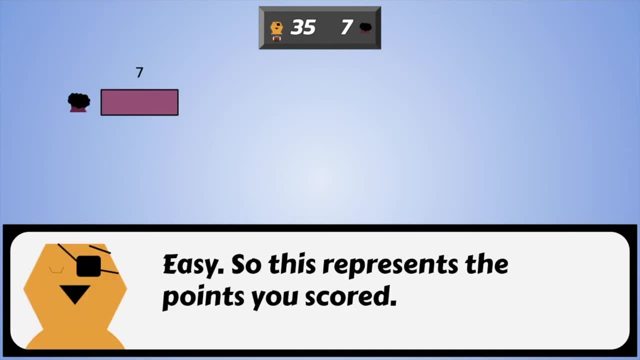 So we'll figure out how many times as much was my score compared to yours? Sure, Start by drawing a small bar to represent the 7. Easy, So this represents the points you scored. Good, Now we can compare that to the points you scored. 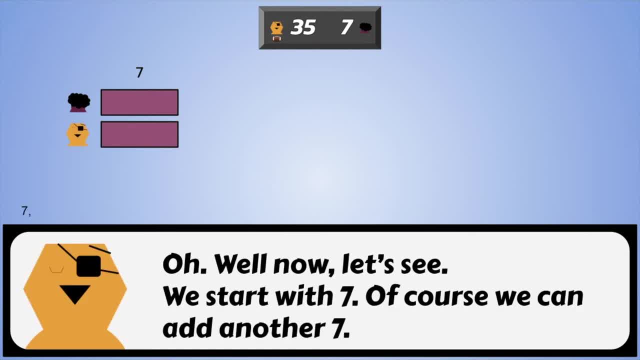 How many times do we need the number 7 to reach 35?? Oh well, now let's see, We start with 7.. Of course, we can add another 7.. Let me draw this rectangle. That's 14 so far. 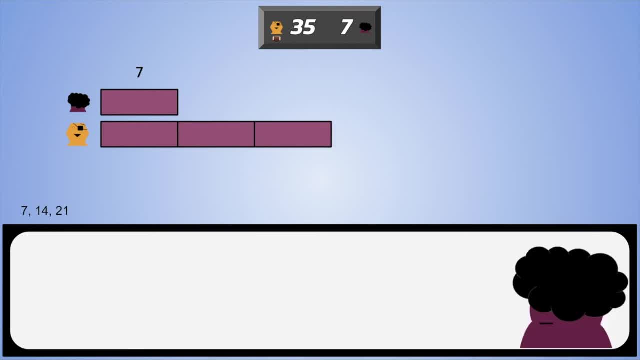 Okay, draw another bar, 7.. Oh, that's only 21.. Maybe one more will do it. No, That's only 28? Sheesh, Okay. okay, One more bar, and we finally made it to 35.. Good, So do you know how to read your model? 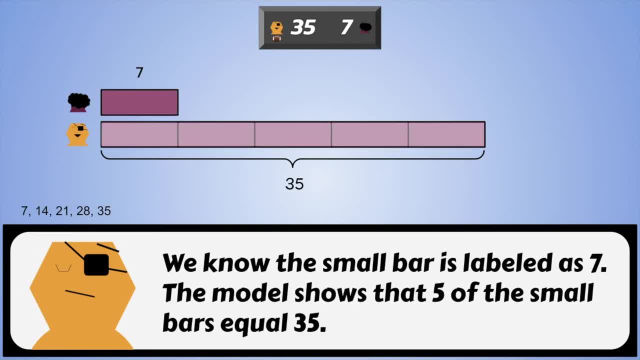 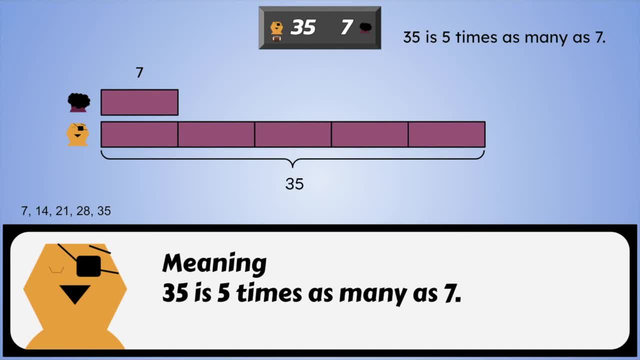 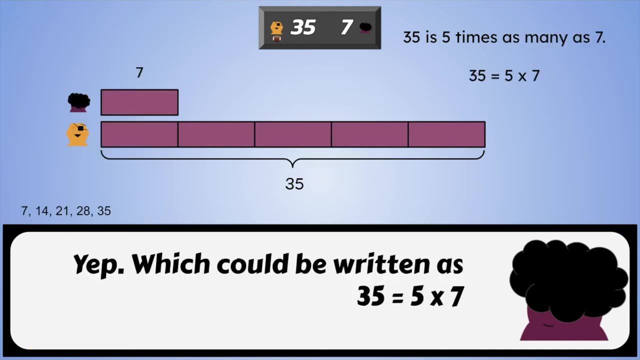 We know, the small bar is labeled as 7.. The model shows that 5 of the small bars equal 35. Meaning 35 is 5 times as many as 7.. Hey-oh, Yep, Which could be written as: 35 equals 5 times 7.. 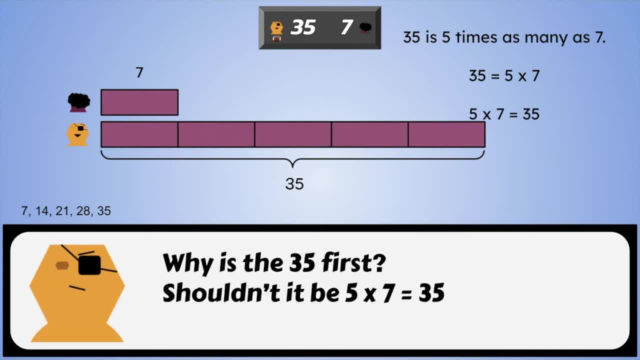 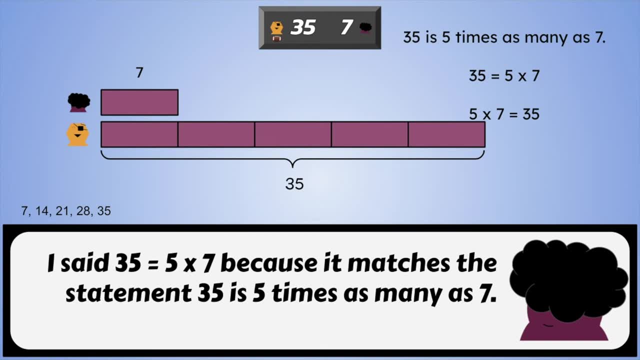 Why is the 35 first? Shouldn't it be: 5 times 7 equals 35?? Either one, It means the same thing. I said 35 equals 5 times 7 because it matches the statement: 35 is 5 times as many as 7.. 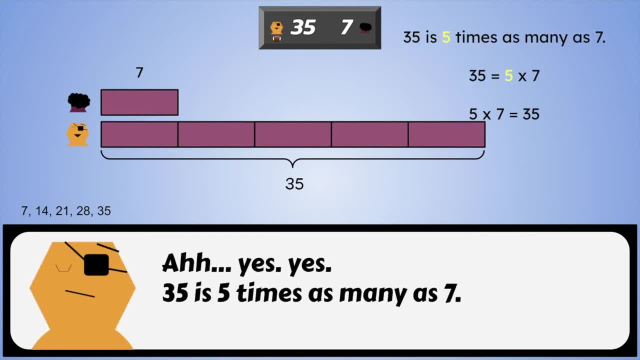 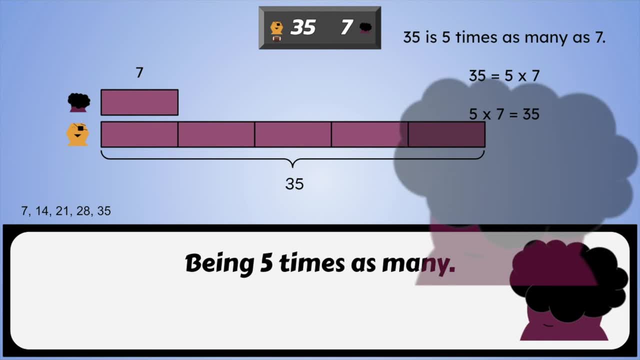 Ah, yes, yes, 35 is 5 times as many as 7.. Indeed, Indeed, Yes, I see you 35. Being 5 times as many. Wow, I really had 5 times as many points as you, huh.